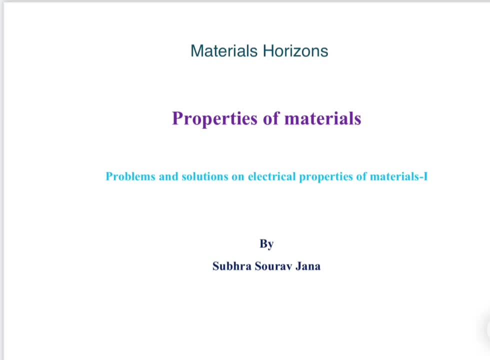 science and also beneficial for other branches like electronics, mechanical physics, etc. It is also helpful for competitive exams like GATE. So today I will also talk little bit about theories while solving problems. So, without wasting further time, let us solve. 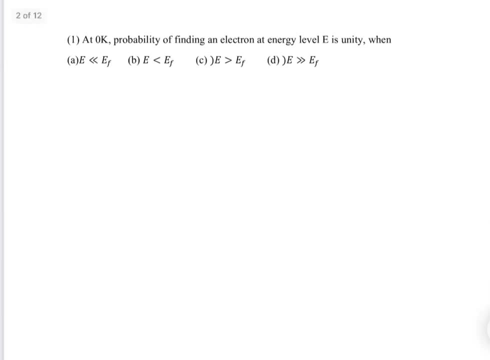 some problems. So it is the first problem. So at 0 Kelvin probability of finding an electron at energy level E is unity. When So we have to find the conditions, Well, the occupation probability is unity. So highest field energy at 0 Kelvin is Fermi energy That we already know, given by 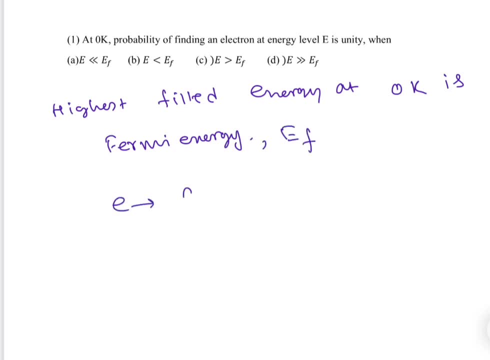 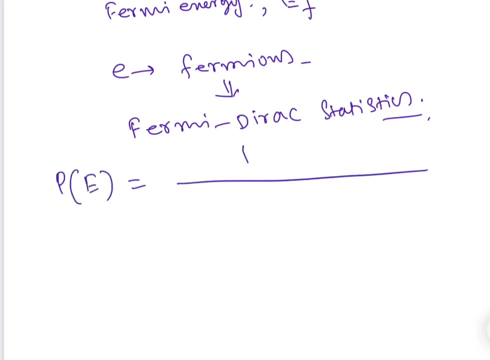 EF Electron is fermions, So it is most obvious It follows Fermi-Dirac statistics. Hence the occupation probability can be given by this equation: E minus EF, by E F, So EF minus EF, EF minus EF. 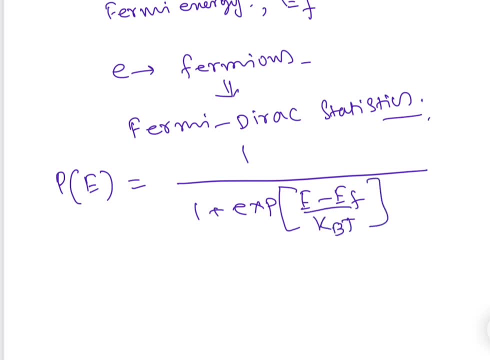 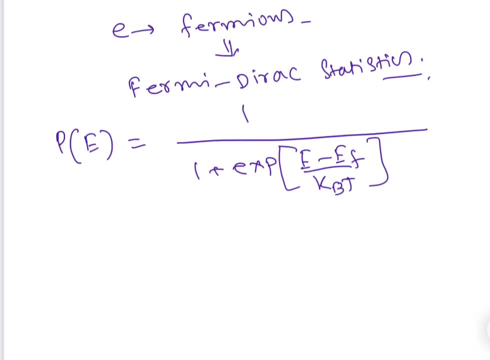 So EF minus EF divided by kB T, kB T or kT, whatever, I sometimes prefer to write kB. So by this equation, if we plot the probability function at 0 Kelvin it will be like this: At Fermi energy it becomes 0. Right Above Fermi energy, it becomes 0. EF will be equal. 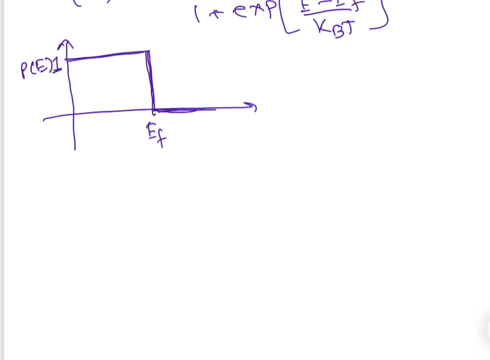 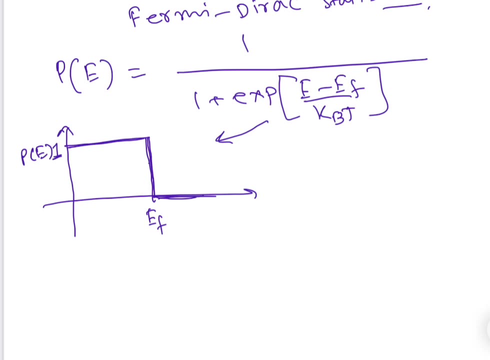 below Fermi energy. it is unity. So by that equation we can find this. But if you increase the temperature it will come like this: More increase it will come more flat. So it is suppose T2, it is T1 and this is 0 Kelvin. Then we can easily write T2 greater than T1. 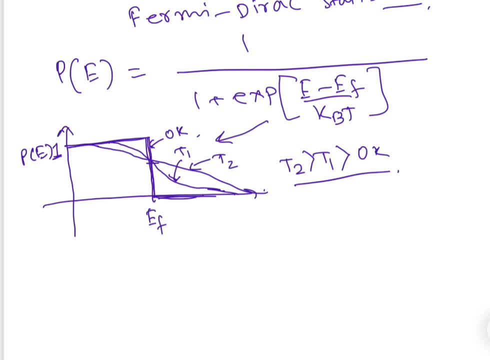 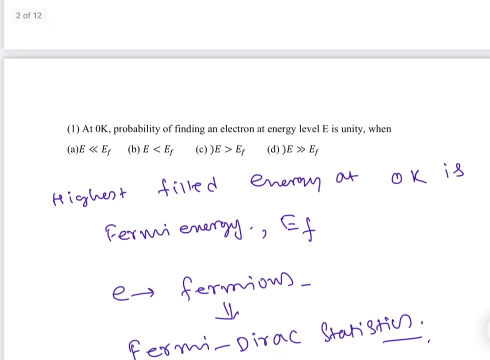 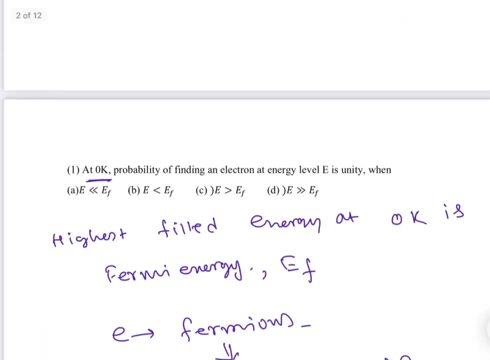 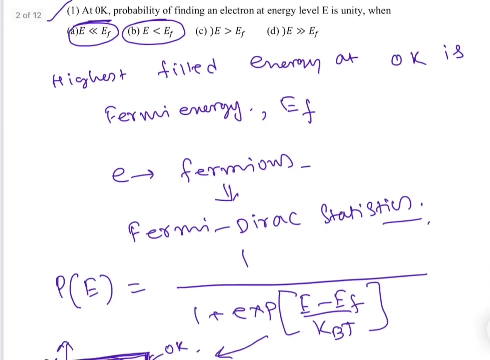 greater than 0 Kelvin. So we can easily find that by this 0 Kelvin, because the problem was at 0 Kelvin. So the unity is below EF. So it may be E less than less than EF, it may be E less than EF. So these two ones. Let us go to the second problem. 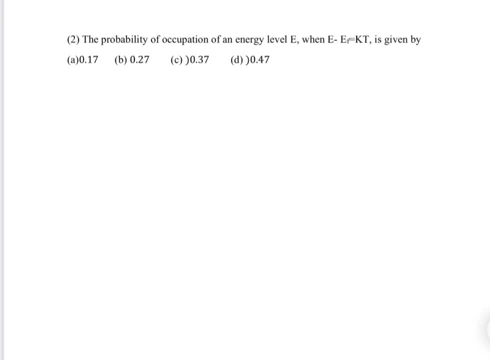 The probability of occupation of an energy level E, when E minus EF, equal to KT, is given by this. So here also, similarly, like the first problem, we will first write the probability of occupation. So it is better to remember this formula, because we will, we will use. 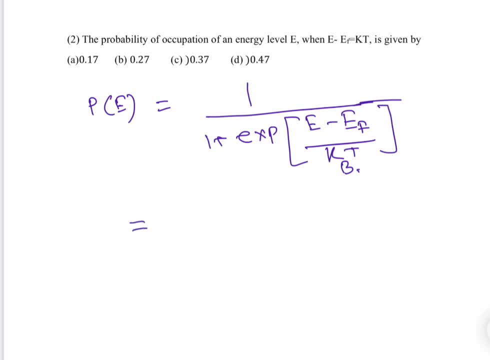 quite a lot. So it is given that E minus EF is KT or KBT. So we will put it here, Then we will. we can write exponential: This is 1, right, This is 1.. So it means 2.7 around. 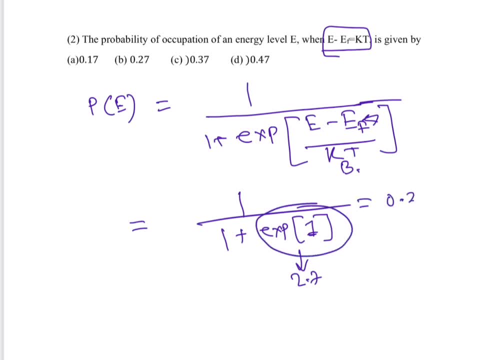 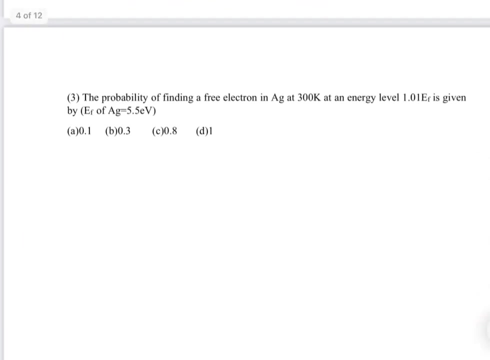 this value. So ultimately it will come 0.27.. So the answer B. So obviously this is T greater than 0 Kelvin, because at 0 Kelvin above a firm energy there is, we cannot find the electrons. So let us go to the third problem. 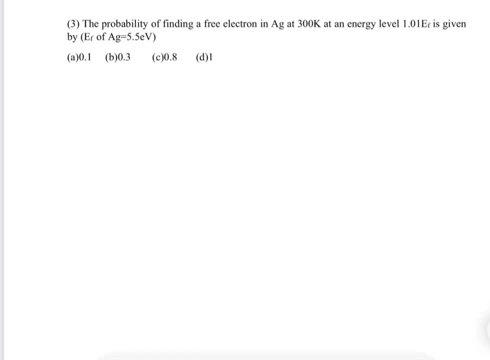 Third problem: Here we have the probability of finding a free electron in Ag at 300 Kelvin at energy level. This is given by okay. So here also we have to find probability of finding free electron. So we have to again find PE. So let us find it Again. we will write first. So if you 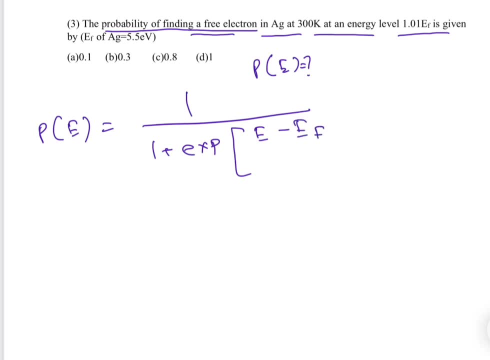 write it again and again, then you can easily remember this formula. So here E is given by, So first suppose EF. I am writing 1.01 EF minus EF. See, it will be like 0.01 EF. okay, 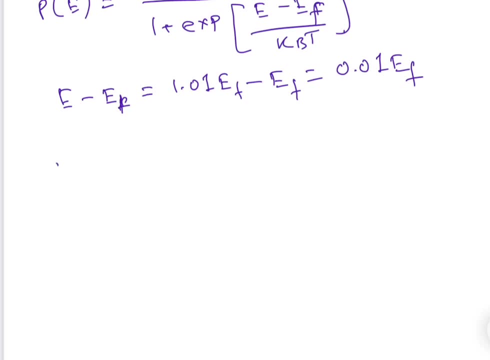 See, if we simply put it in the equation: So 1 plus exponential 0.01 into 5.5.. So sometimes it is better to remember the energy covariance. So then this real of EF will be 1.01 EF minus 1.01 EF. So here is the eF. So here if you want to compare, 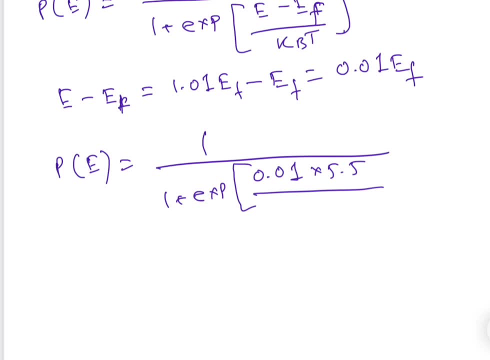 the higher in coefficient. this will be about mod副 So 1 plus exponential 0.01.. So the average eventually gets to be 1.01 in square chakra k, So this will be 2.01 into 5.5 square cœur. sexy for some of the other half value of the. 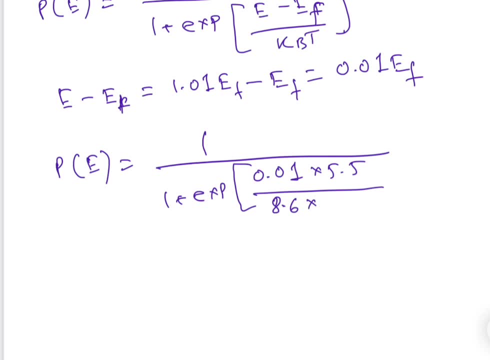 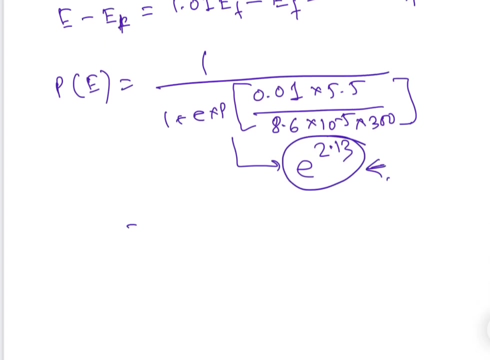 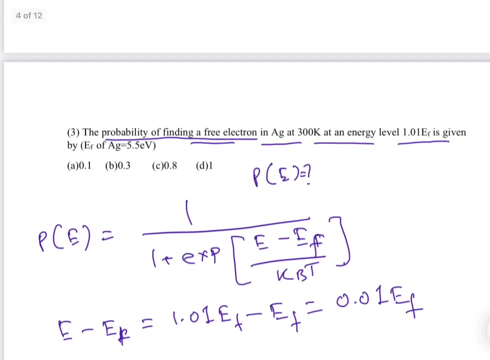 a Boltzmann constant in electron volt. it is given most of the time but still for ease of solution, okay, so ultimately it will come like e to the power 2.13. I have calculated it already so it will come like. sorry, it will come like 0.1. so we have it in a if it is. 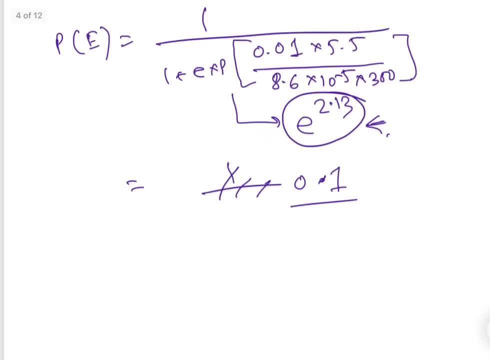 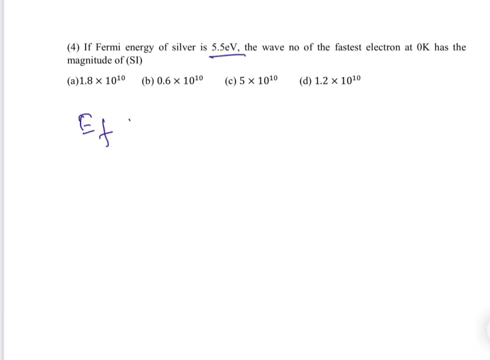 in percentage, then we will simply multiply it by 100. okay, easy, so we will go to number 4. so here, if Fermi energy of silver is 5.5 electron, so EF is 5.5 electron volt. we can simply make it in joule 5.5 into 1.6, 10 to the power minus 19. this is charge of silver. 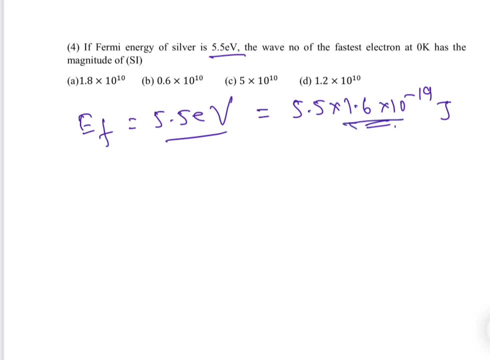 okay, Single electron, so it is better to remember this one: 1.6, 10 to the power minus 19 anyway. so this wave number is given by K. we know fastest electron, 0 Kelvin magnitude, so I do not need to see everything. so here what they want, they want wave number. right, so we know. 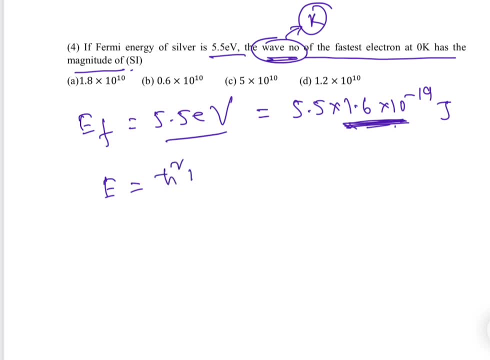 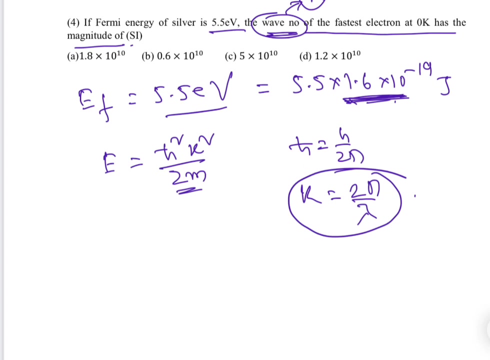 by free electron theory, E equal to h cut square, K, square by 2.. And the h cut is h by 2 pi. right, and we know K is also equal to 2 pi by lambda. however, this is not required here because they are not asking this if electron has a wave property. 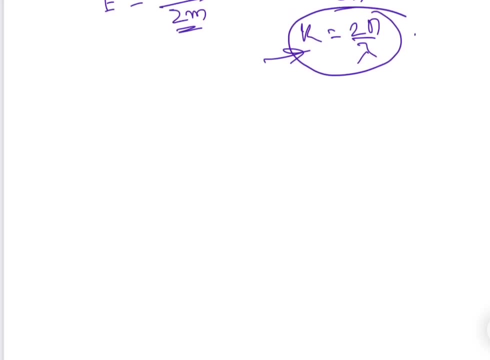 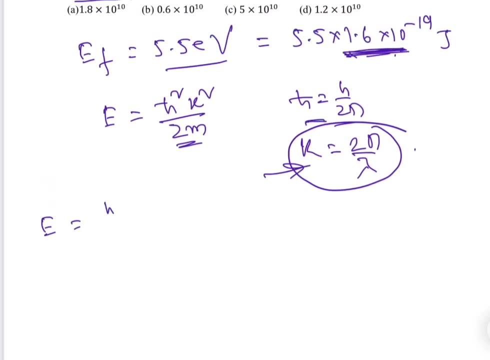 so that is why wave number is coming. so by putting this we have, by putting this one, we have h square by 4.3.. Okay, 4 pi square into K square by 2 m. okay, next we have equal to h square, K square by 8 pi. 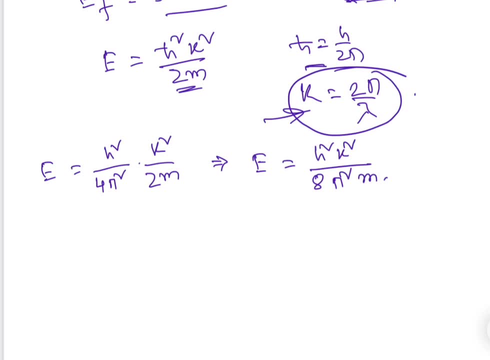 square into m so we can have the K value, because at last we want the K right. so this will be 8 pi square, m into E by h square and this is equal, to just simplify it, A, 2 and a, and if we put the value of everything like here, h is equal to just. we will put here: 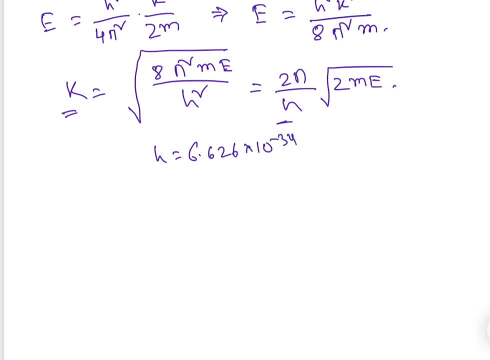 6.626 into 10 to the power minus 34. It is better to remember, or else sometimes it is given he is just Planck's constant and M similarly. M value is 9.11, 10 to the power minus 31 kg. 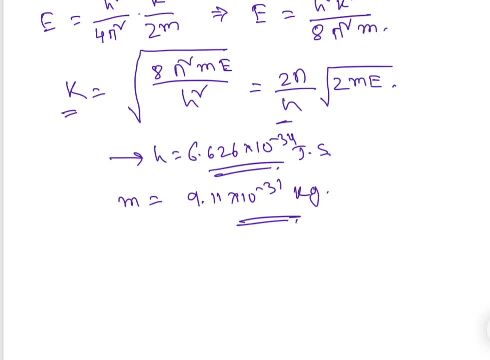 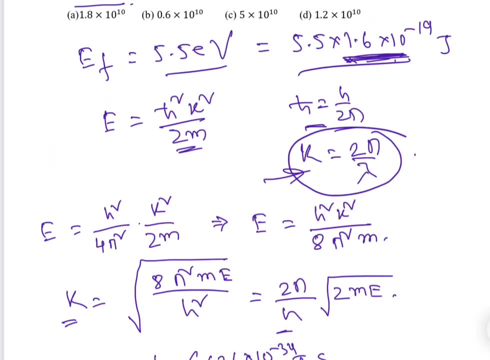 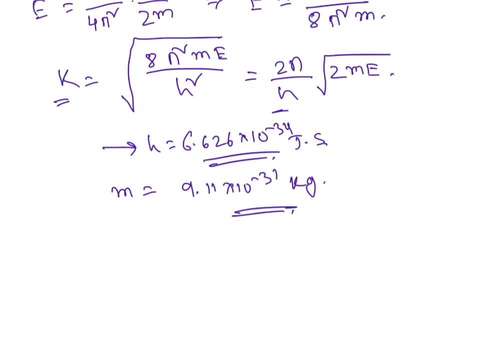 Okay, Okay, Okay, Okay, Okay, Okay. And e we have already written here. So if we put so, this is in Fermi energy. So ultimately, what we have, if we put all the values, we will have k equal to 1.19 into 10, to the power. 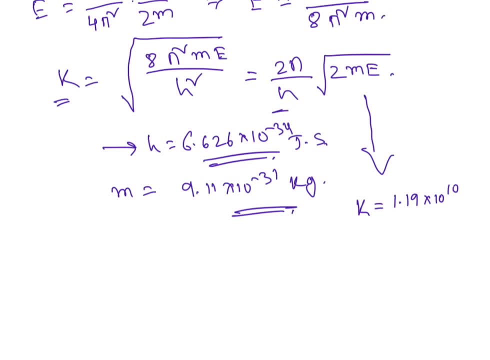 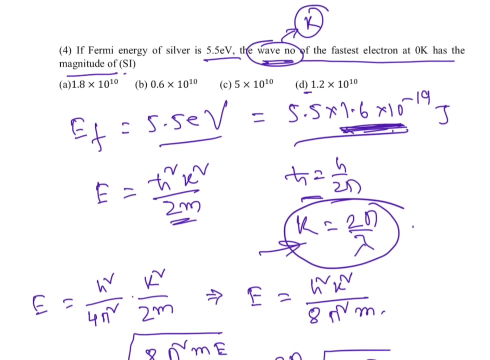 10. Obviously, b causes about unit, So wave number meter, because everything we have put in SI, So it will be meta inverse, So we will see which value is close to it. 1.19 means it is close to 1.2.. So the correct value is 2d. right, So let us move to the 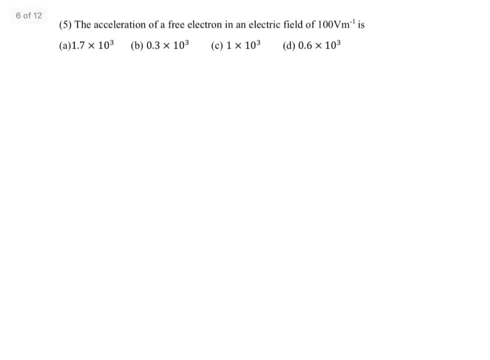 next problem, problem number 5.. The acceleration of a free electron in an electric field. The force experienced by a electron is given by e into e. e is the applied field, into e. sorry, e is the electrical charge, But in classical mechanics or Newtonian 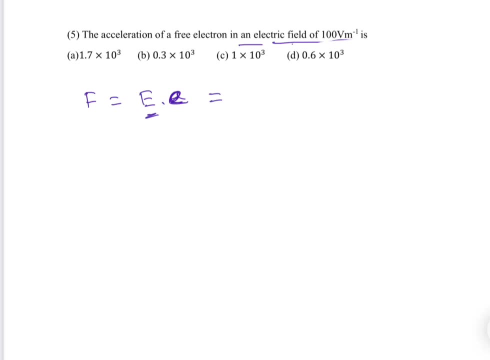 mechanics. we can also write it. If I consider electron as a particle of mass m, then we can write it m into a. that is acceleration. So if I consider electron as a particle of mass m, then we can write it e into a. that is acceleration. So if we equate these two, then 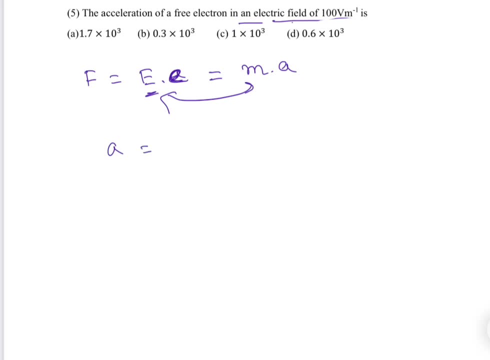 we can find, sorry, a equal to e into e divided by m. Just putting the values here, 100, because we have 100 volt per meter into electron charge, we know 10 to the power, 19 divided by electron mass. So that is fine. If we have a electron charge we have 10 to the. 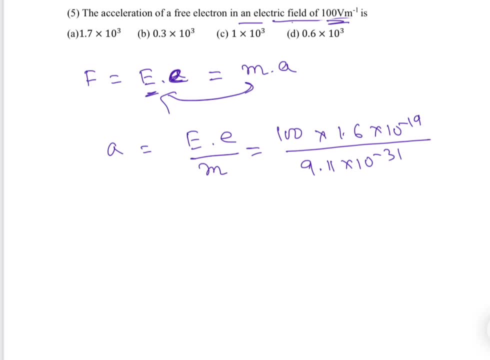 mass. It is better to remember those things like electron mass, electron charge, Planck's constant, because they are helpful in many cases. Sometimes it is not given anyway. So we can calculate it And we can find 1.7 into 10 to the power, 13 meter per second square. 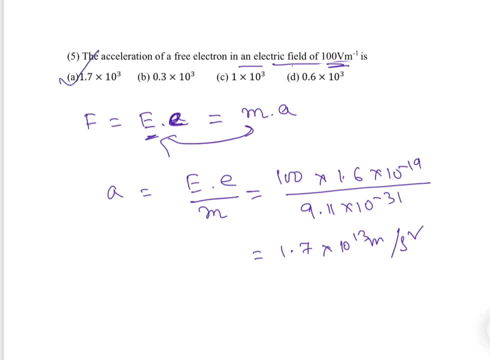 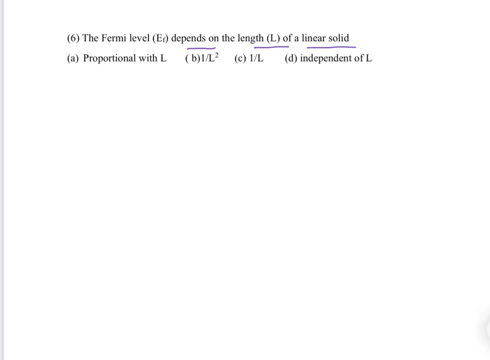 So 1.7.. So this will be answer A. Let us move to the problem 6.. The Fermi level of air depends on the length, So Fermi level is actually an energy level. So that is the highest energy level occupied. 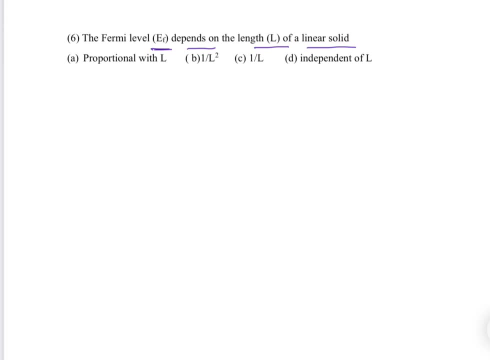 by electron at 0 Kelvin. So there is no dependence of length of the solid, So at least at the bulk level. So that is why it is completely independent on L Right. So problem 7. Morph: At these temperatures the collision time of electron scattering in. 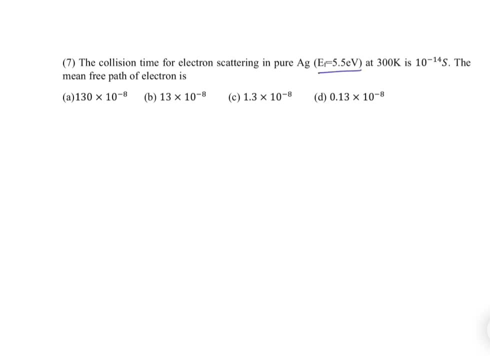 pure a g where the EF is like this, So at 300 Kelvin is a. 300 Kelvin is 10 to the power minus 14 second. The mean free path of electron is. So we have to find the mean free path. So before that I will just talk here little bit. see the collision time they are given. 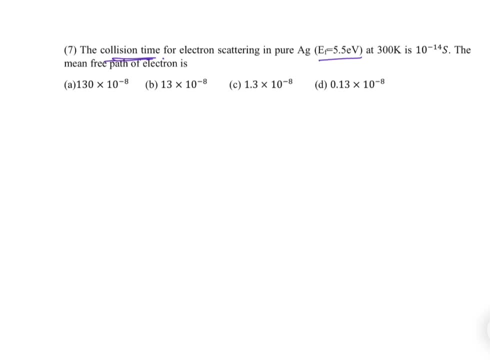 collision time means electrons are colliding right. So electron is colliding with what? so at very, I mean at lower temperature near 0 Kelvin. So what will happen? so as the temperature is increases, is increased above 0 Kelvin, the phonon modes are activated. I mean lattice. 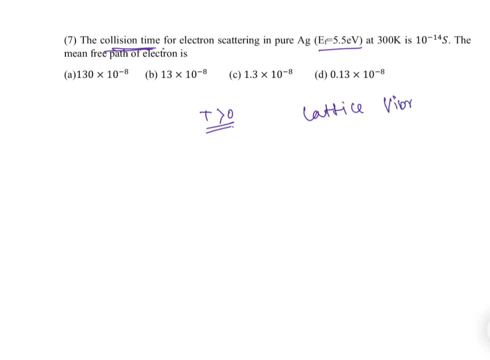 vibration, this lattice vibration, this quantum of lattice vibration is called the phonon. So above 0 Kelvin lattice vibrations are generated and that produces phonons. I mean quantum of lattice vibration is called phonon. So this phonon will scatter electron. ok. 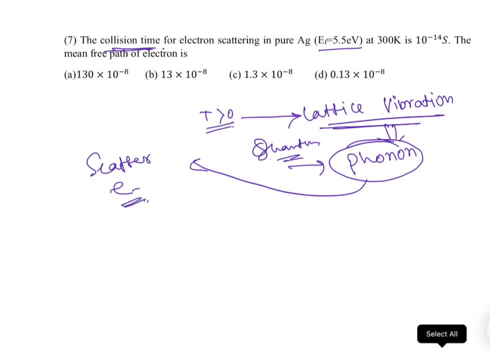 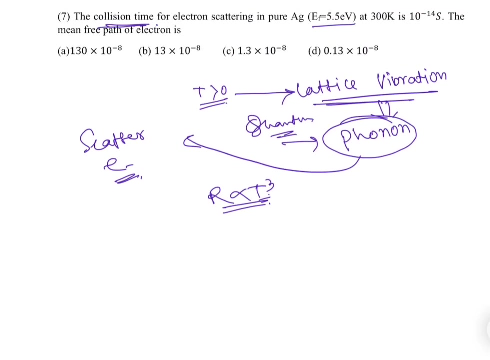 So this phonon will scatter electron, ok. So that is why roughly we can say at lower temperature resistance that is just t cube, t is temperature. the resistance increases with temperature, ok, as the mode scattering happens. So between 2 collisions, average time between 2 collision is given by tau that. 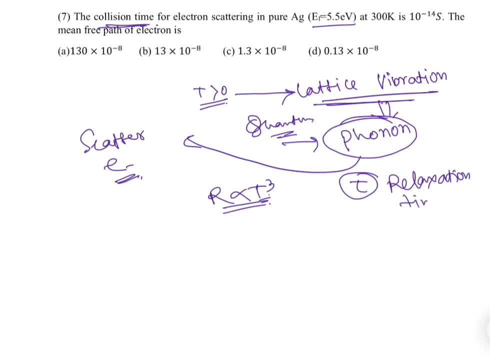 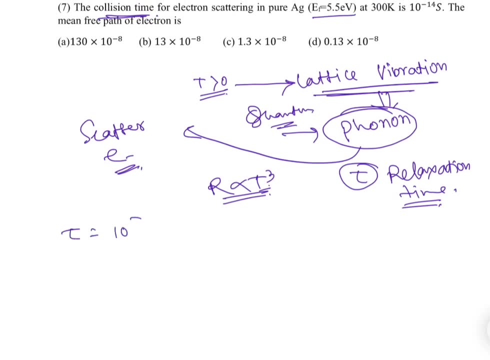 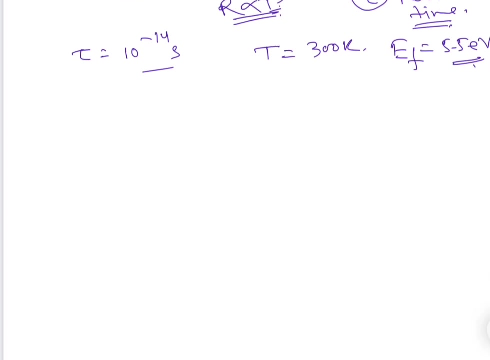 is relaxation time, similar like gas molecules in a box. So this tau is given here, 10 to the power minus 14 second, and T is 300 Kelvin and EF is 5.5 electron volt. we can convert it in joule, So what they want. they want mean free. 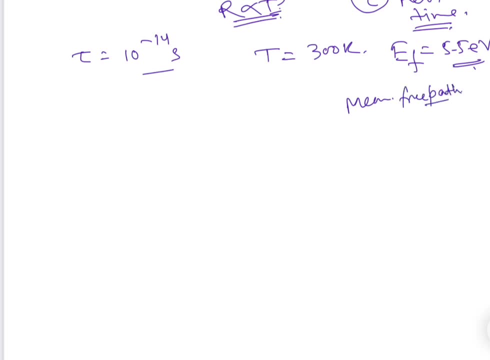 path. So mean free path means the distance covered by an electron between two collisions. okay, so between two collision, time is tau. if we multiply it by its drift velocity or velocity, then we can find the mean free path. So we need the mainly velocity, right? how? 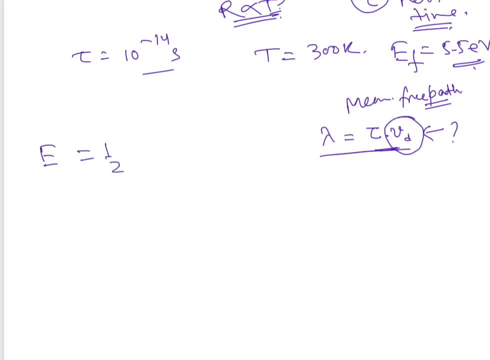 will I get? so we know that energy is half mb square. classical mechanics is the velocity, m is the mass of the electron and E is energy. So most of the electrons which are in Fermi energy will take place, Thank You, in conduction. So they will move. So that is why this energy we will put as EF right. 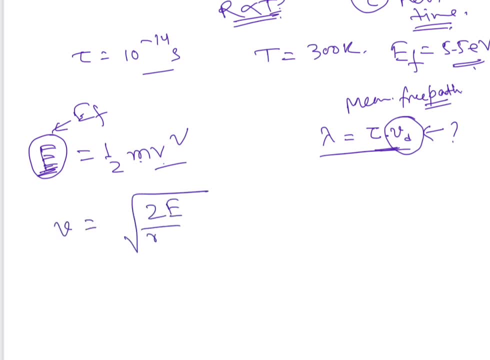 So V is actually 2E by M. Again, we will put the values 2 into 5.5 and convert it in joules, So 1.6, 10 to the power minus 19.. That is coulomb. I mean. this is the charge of an electron and the 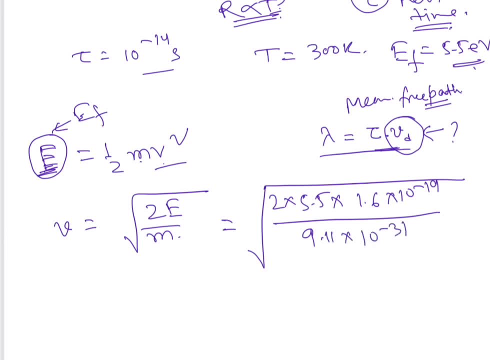 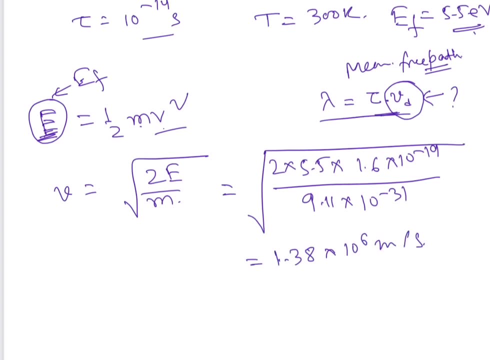 mass of helium: 9.11, 10 to the power minus 31 kg. So ultimately it will come meter per second. So it will come 1.38 into 10 to the power, 6 meter per second. It is not yet done, So 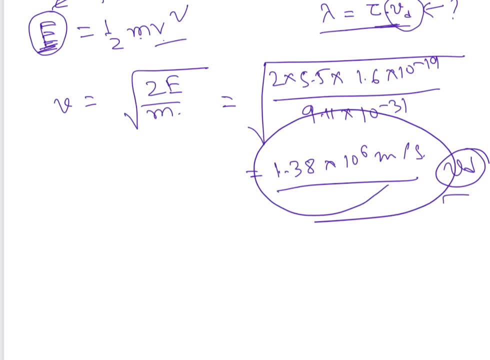 we got the VD or drift velocity. So if we want to have the mean free path, that is this drift velocity into tau, So this drift velocity is 1.38 into 10 to the power 6 multiplied by 10 to the power minus 14.. So ultimately it will come 1.38 into 10 to the 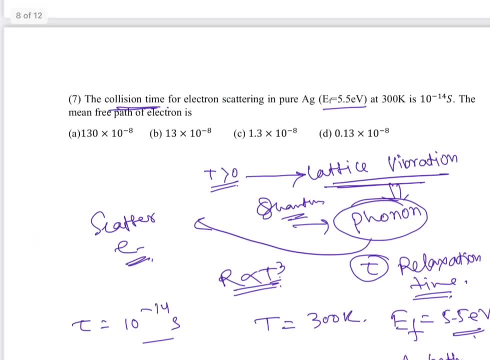 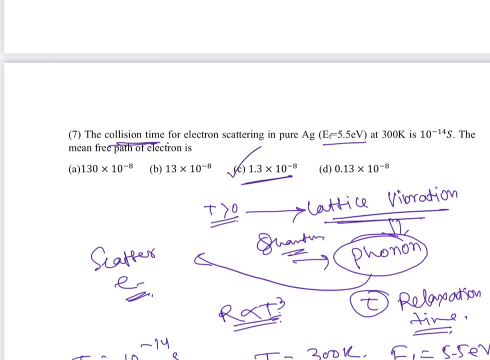 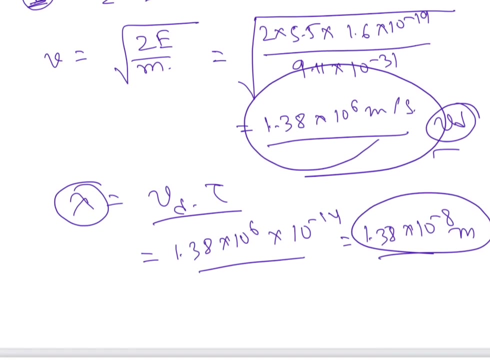 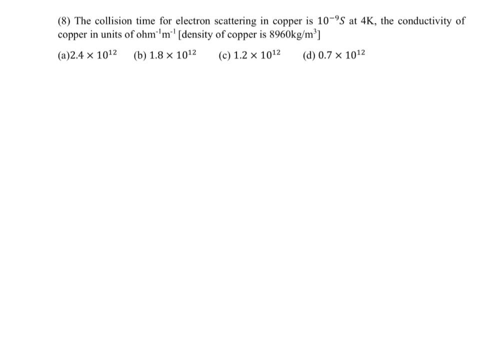 power minus 8 meter. See which answer we are close to. Yeah, this one Yeah. So answer C is correct, right? So let us go to problem. The collision time for electron scattering in copper is 10 to the power minus 9 second. So 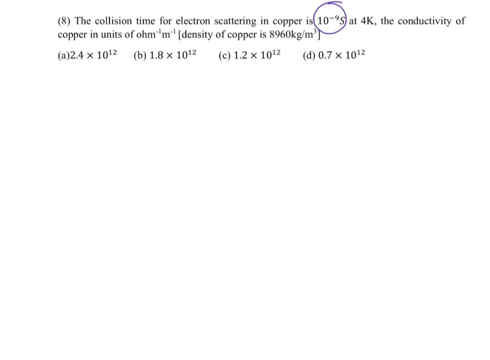 again, tau is given at 4 Kelvin. The conductivity of copper in units of ohm inverse. Ohm inverse means actually cement. Sometimes cements are given Okay, So density of copper is given Okay. So tau is 10 to the power minus 9 second 4 Kelvin. This is not. 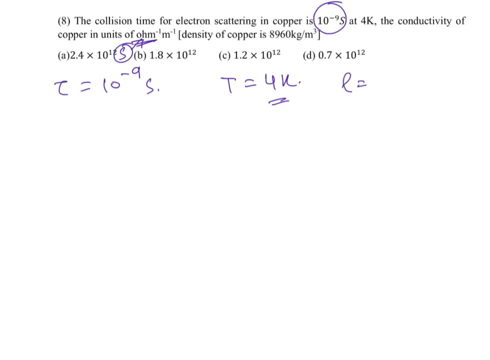 required, I guess. So density, I am putting it like d density, 8960 kg per meter cube. I put everything in SI, always, So by Drude's model, sigma equal to sigma is electrical conductivity. This is electron. 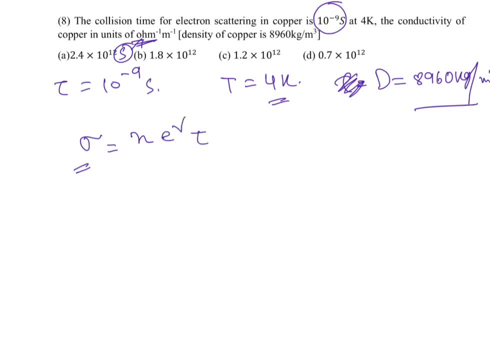 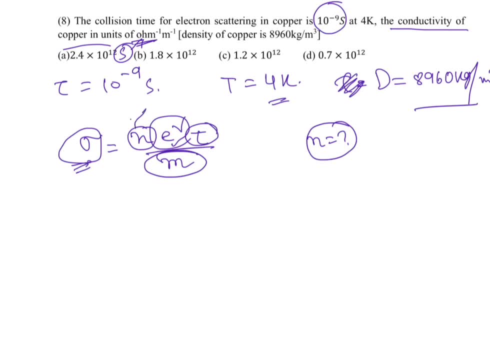 So we are putting conductivity n. So we are putting conductivity n E square tau by m, And here we do not have n, But rest is given. So for n. how will I get n? So the catch. 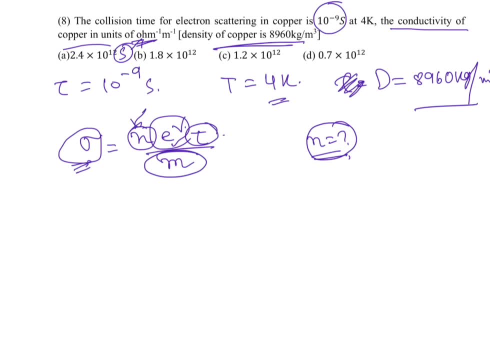 is this density? Okay? So what will happen? So we assume that copper is given one electron, one valence electron, to the conduction mechanism. So ultimately, so one mechanism means for each mole. they are giving Avogadro and Yuze, So every mole is given. Now, if we have this, 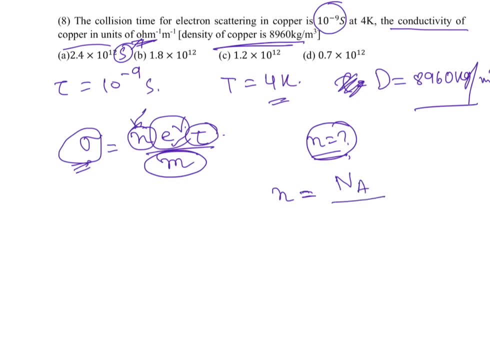 one valence electron is given to the conduction mechanism. So ultimately, one valence electron. so one valence electron is given. So ultimately for each mole, they are giving Avogadro and number of electrons. but if we consider each kg or by each gram, whatever, so that is for. 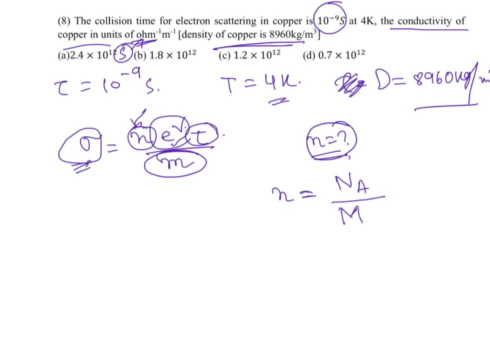 that we have to divide it by molecular mass of copper then. but ultimately here actually this n is per unit volume, I mean in SI per meter cube. so that is why we have to multiply it with density of copper, this one right. so by this trick actually we can get what is. 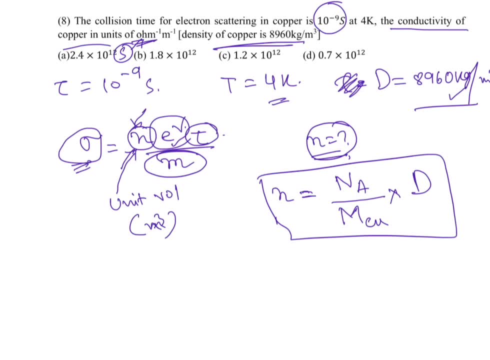 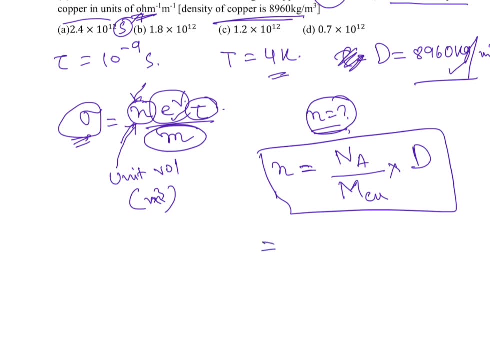 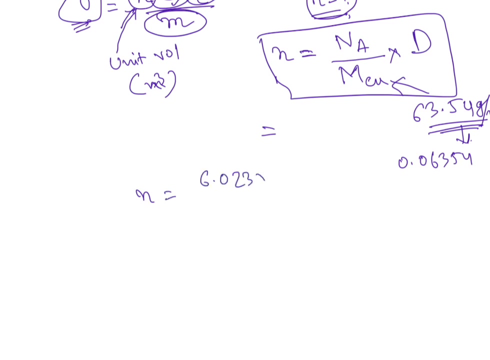 the number of electrons right. so, or electron concentration per unit volume meter, cube and m of copper is 63.54. it is in gram per mole. so ultimately we have to change it in SI, so that will be 063.54.. So let us put the value here n equal to 6.023 Avogadro number. this is just simply. 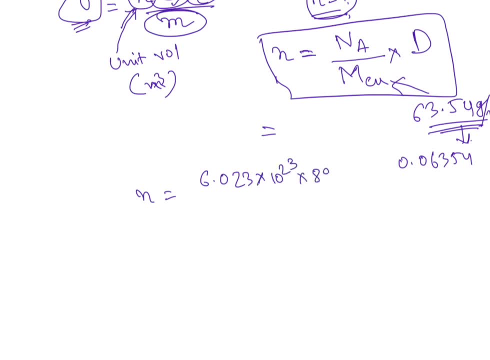 Avogadro, number 10 to the power 23 into 8960 divided by 0.06354, so it will come like 8.49 into 8960.. So this will be 1000 into 10 to the power 23 into 8960.. 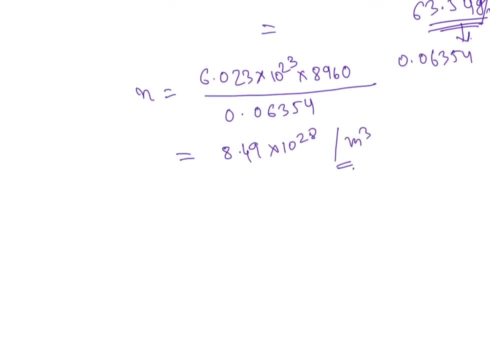 So this value is equal to 6.023. Avogadro number 10 to the power 23, into 8960.. So now, if we substitute this in the form here, we will get the sum of this, we will get 4.Hey, that is the quantity. so what we are going to do, and that is we are going to stress- the electron concentration into the form here. so again, the constant of electron concentration will be 10 to the power 23, so it is also equal to this. so we will just simply put in the. so what we have written in the Drude formula: n? e square tau divided by m am. 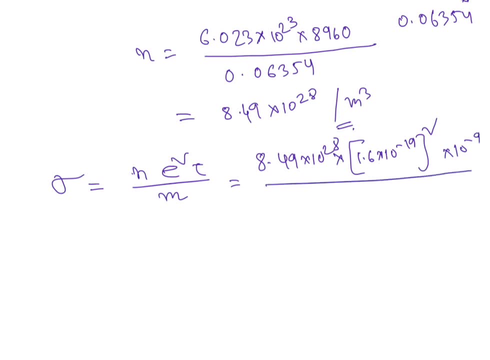 So here we will simply put this 0.98 into the 28, into electron charge, that is 1.610 to the power minus 19 whole square into 10 to the power minus 19.. 9 tau is 9, right. and then 9.11, 10 to the power minus 31 kg. sorry. so what will come? 2.38, i have. 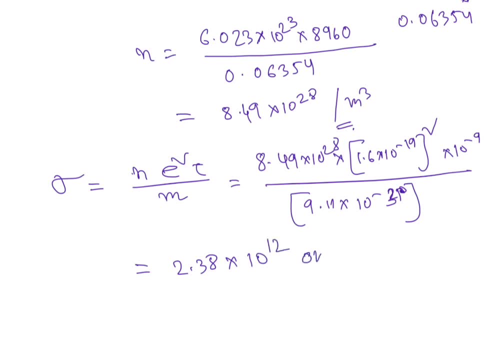 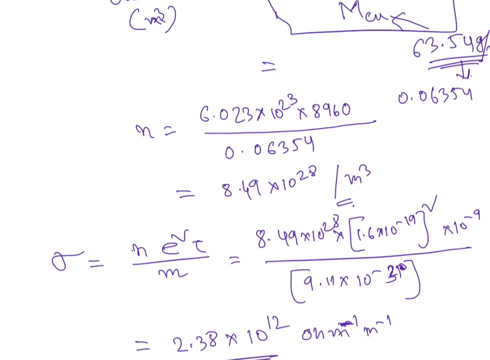 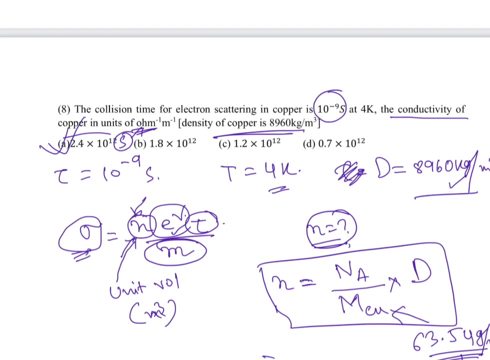 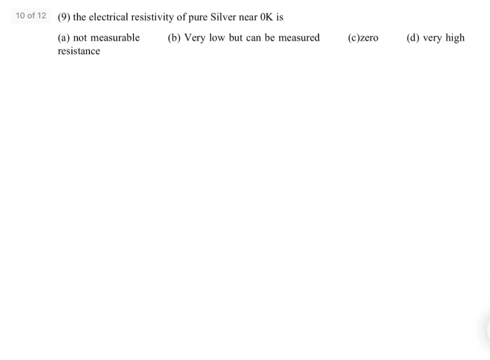 calculated it already. so that is in ohm inverse, meter inverse. so it is close to which answer? 2.38. yeah, so the first answer, so the answer will be a. okay, let's move to the 9. what is so? 9 is like the electrical resistivity of pure silver, near zero kelvin. 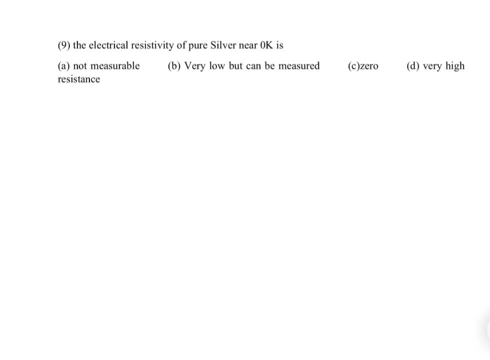 okay, so we know that the four where i have already told that above zero kelvin the lattice vibration increases, i mean phonon modes are generated. so ultimately the elect electrons are scattered and electrical conductivity reduces. it means electrical resistivity increases with temperature. resistivity increases, suppose with cube cubic. so it will be like that. so 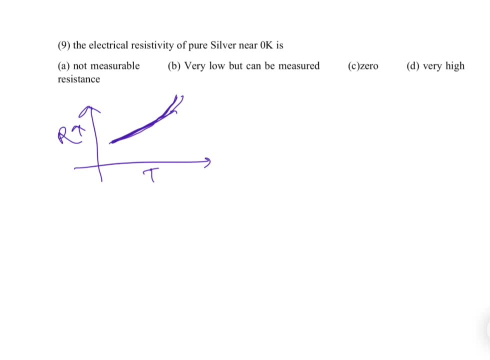 this is resistivity with temperature at lower temperature region, so at zero, near zero kelvin Brisbane. so it will be very low but obviously measurable. very low but can be measured, this one. so it will be b.0, 0. it will have certain values because of that lattice vibration. okay, so let's go to number. 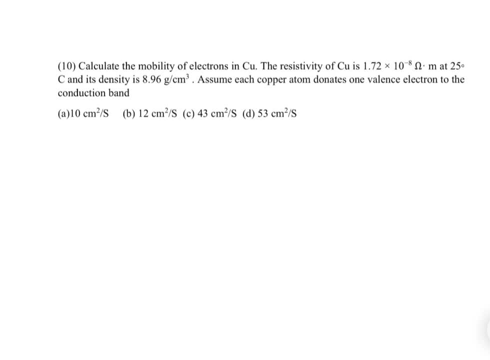 10 calculate the mobility of electron in copper, the resistiveuffs active number 10 will have some kind values. because of that lattice vibration, number 10 is a very small amount. arguably you can. you can do it like you do with any object, like epinephrine, or you can. 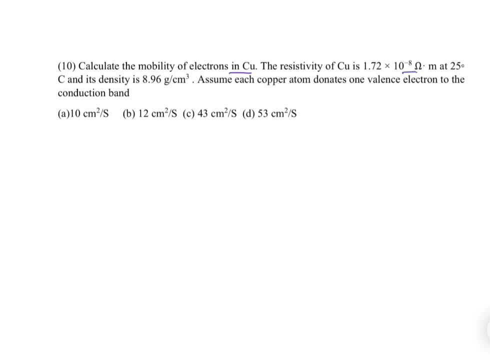 never get it. so so what will i do that? this is the takeaway, low, but can be measured this: the resistivity of copper is 1.7. okay, so density is like that. again, density is given here. that means that thing we have to do, i guess. assume each copper atom donates one valence electron. 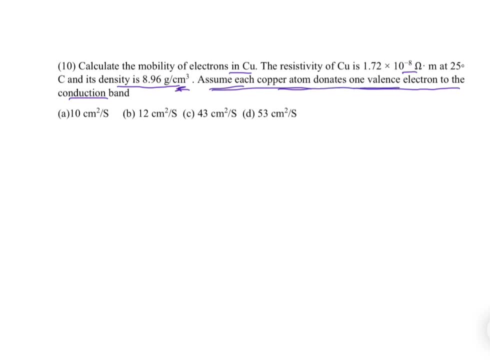 see here, each copper atom donates one valence. here it is given. but the previous two, previous problem, it was not given. so we have to assume, in that case, right, okay, so first of all, the mobility we know. so mobility we have to define. so what is mobility? first of all, the mobility is actually. 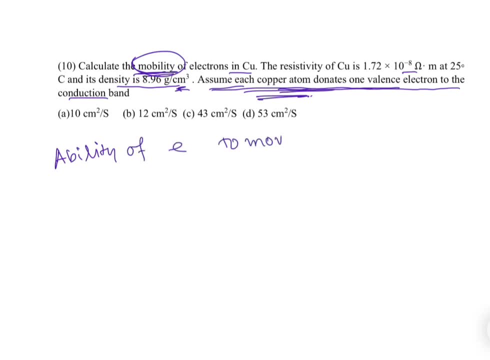 ability of electron to move, here for electron we are considering. so that is why electron i am writing. so this mobility is given by, sorry mu mu, is given by v, by e, velocity of electron, here everything electron. so i am writing here always electron, and e is the 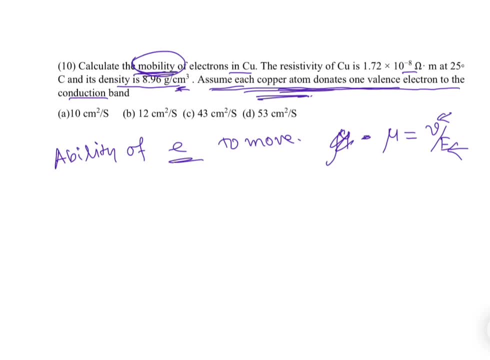 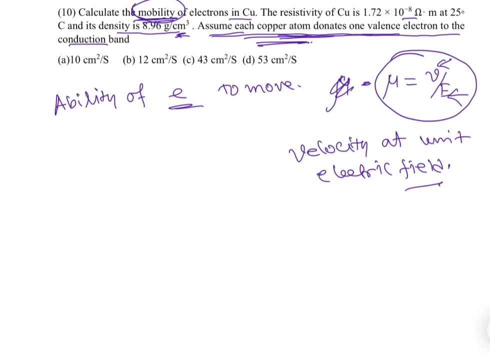 um, um, um electric field. so it can be defined in other way, also velocity at unit electric field, okay, velocity achieved at unit electric field, like that. so so first of all, uh, we have to get the mobility. so for that conductivity sigma is ne mu, mu is mobility, n is the electron concentration. so now the sigma is again ones by rho, so mobility is one by rho, n into e, n into e, okay, by the mu is mobility number, then it is going to be 1 by rho and us mu, mu, also mobilityата type. so that is the electron concentration. so now then Break Electron Communication. 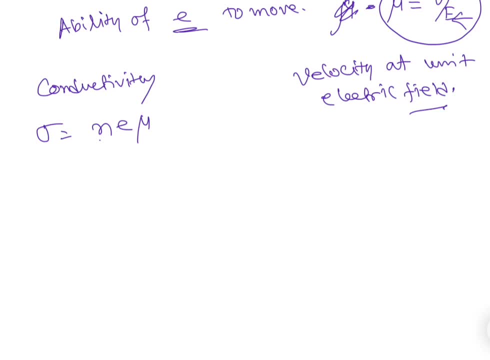 we is the electron concentration consen. the sigma is again won by. so mobility is one by ng, our 120 not, but that is the current 1 by row. so mobility is 1 by row. N in 2 times be in every segment, deh. So now the mane, هذا is� deception. LED andajcs. 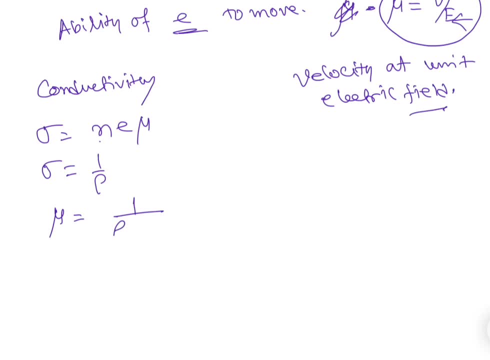 So mobility is one by row N in 2 anding table it is going to be e. one of the like J is equal to power vector monitor. another wave of the effect is no image share, an ideal expression. that number will be negative. okay, By the way, what is this? n Electron concentrations. like the previous problem, 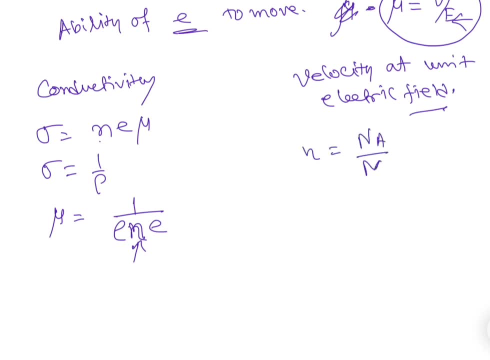 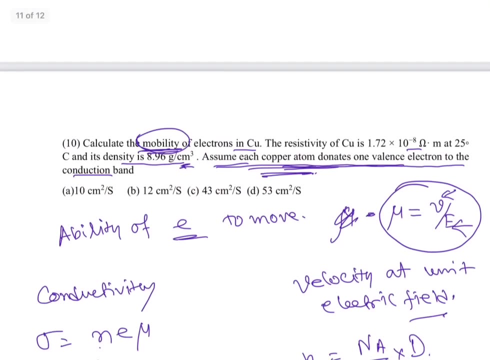 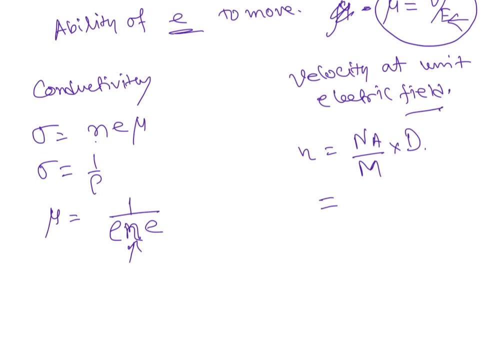 Again, n has to be calculated, like Avogadro number, by molecular mass into density, right? So by putting all the values here we have the values of density and 63.5, like that Avogadro number we know. So ultimately we will get 8.49 into 10 to the power 28,, right? 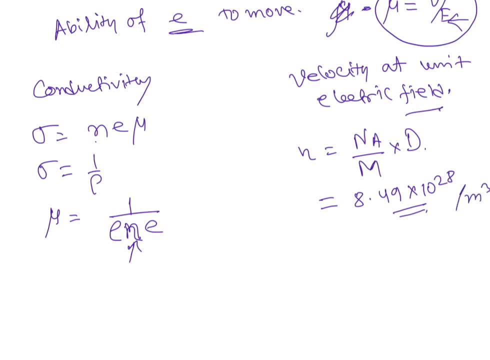 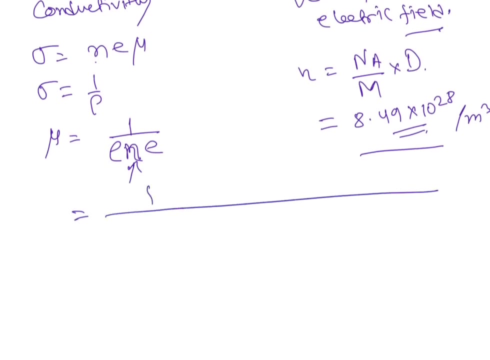 Like the earlier problem, exactly same. So per meter cube, and we have to just simply put here this: rho value 1.72 into 10 to the power minus 8 into 8.49 into 10 to the power 28. 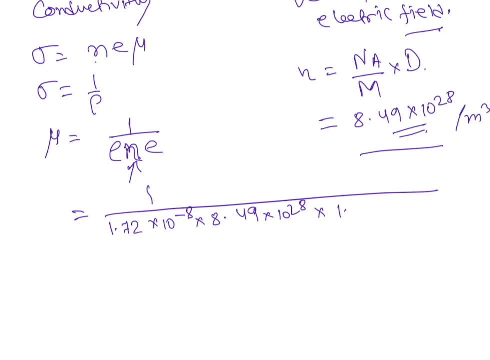 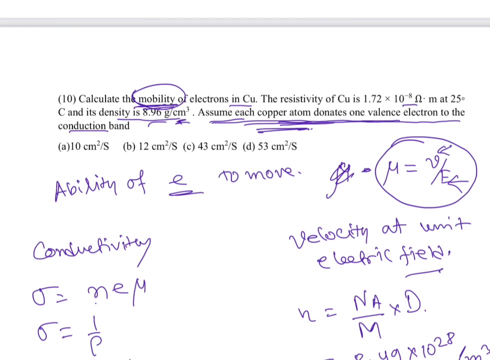 into again: electron charge 10 to the power minus 19.. And everything I am putting in a psi unit. So ultimately we will have 0.0428 meter square per second. yeah, Careful about the unit meter square per second, right, But here we are seeing that these are in centimeters. 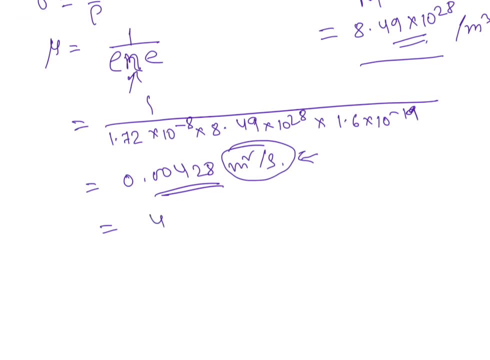 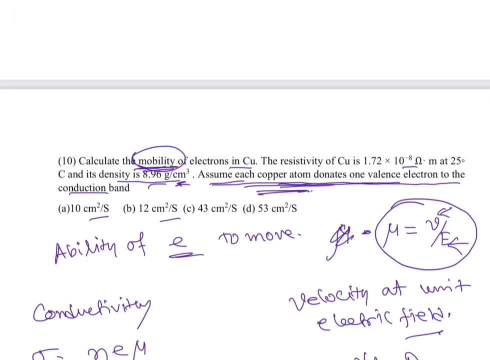 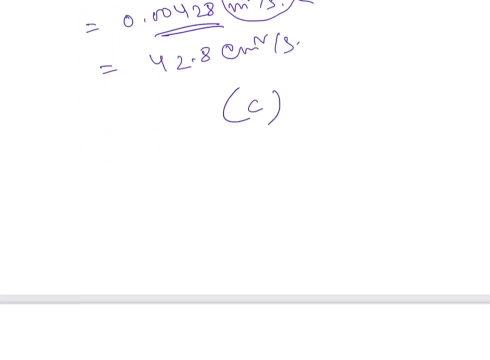 So let us convert in centimeter. It will be like 42.8 centimeters. So it is in. yeah, So it is close. So point C: Right, Yeah, So I will see. So let us move to the number 11.. 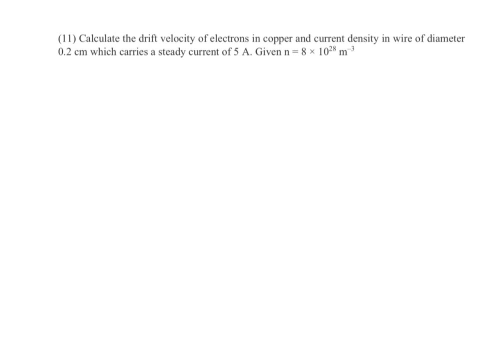 Yeah, So calculate the drift velocity of electrons in copper and current density in wire. So there is a wire which has some cross section. We have to calculate that right. So Ultimately, again, So calculate the drift velocity of electrons in copper and current. 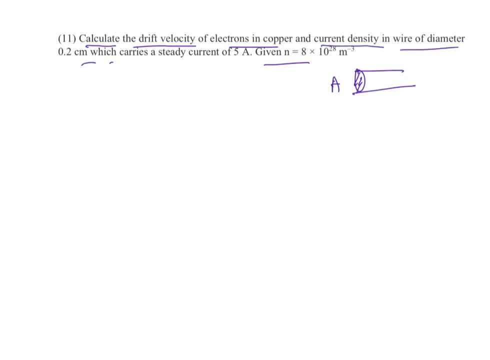 density in wire diameter. So calculate the drift velocity of electrons and current density. Where is okay? So current density we have to get along with drift velocities. So ultimately what will happen? J is the current density Right, So we will have to calculate the current. 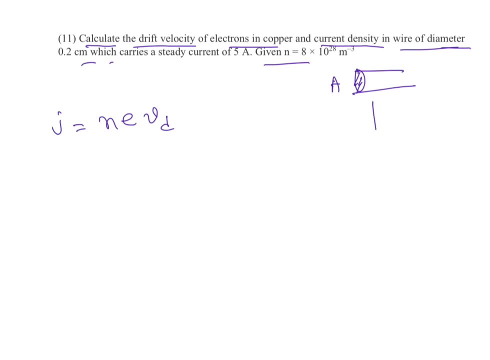 that is navd. and so, because of the collisions, again and again the velocity of electron drops, then again it achieves, the velocity again drops, and between these two collisions- this time is we have mentioned earlier, no, it is just clear idea, clear graphical idea, right. so here j is again. we know i by a and a is cross section. i is given 5 ampere and this a is pi d. 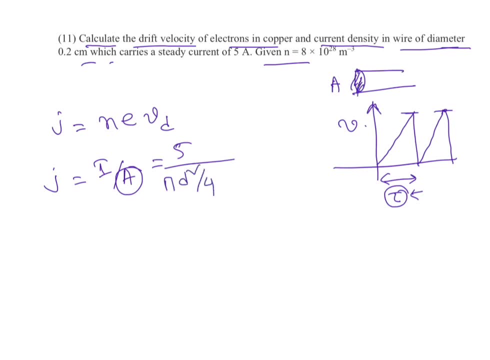 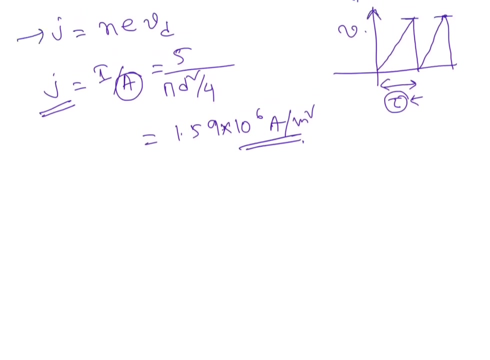 square by 4 because it is just, i mean cylindrical. so we will have 1.59 into 10 to the power, 6 ampere per meter square. so we have got the j, that is current density, and what is the drift velocity? drift velocity we will get from here because 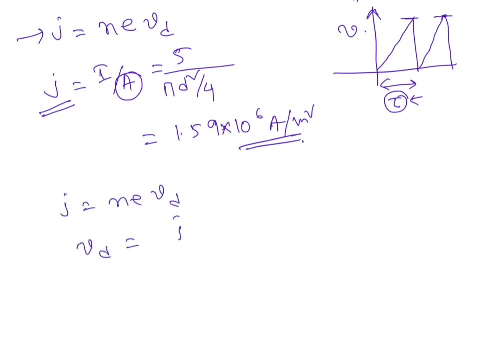 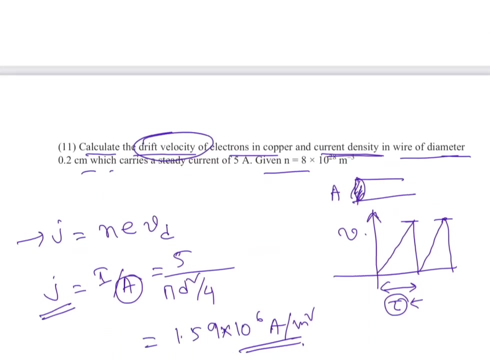 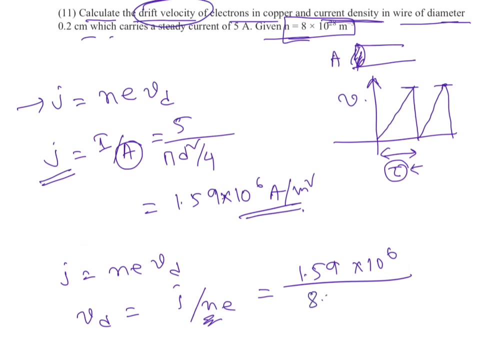 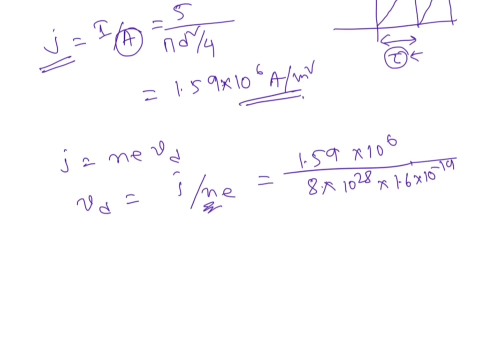 j equal to ne vd, so vd equal to j by ne, right? just put the value 1.59, 10 to the power 6, divided by n in place of n, what we put in place of n, again, this n is given here right. so 8 into 10 to the power 28, 1.6 minus 19. okay, so it will come around. 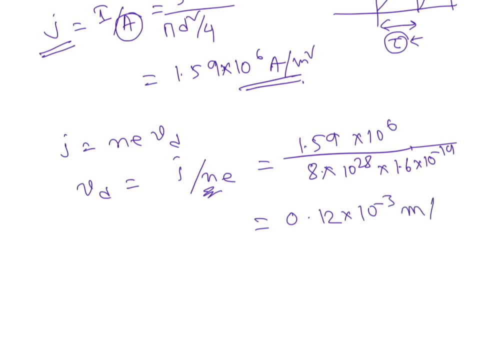 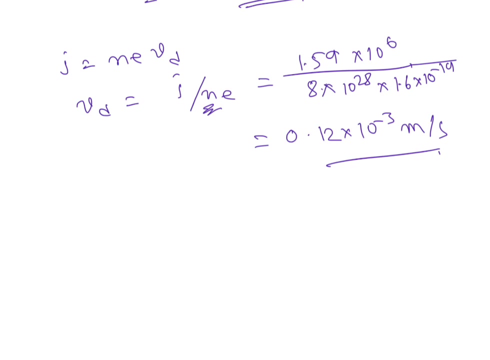 okay, so this is the drift velocity, so this was the last problem. so that is all for today. hope it helped you and i have also planning of bringing some other videos on this, on the theories and also other problems, and thank you for watching it and do subscribe if you like the video and thank you, see you.